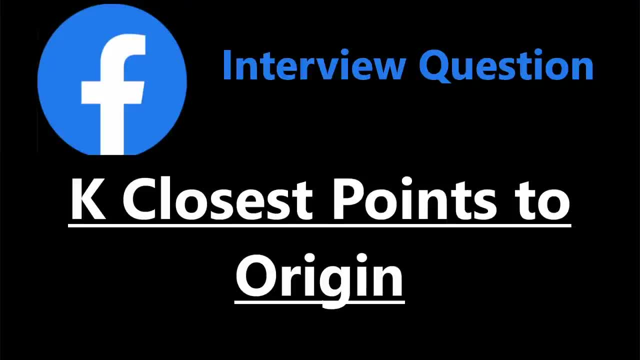 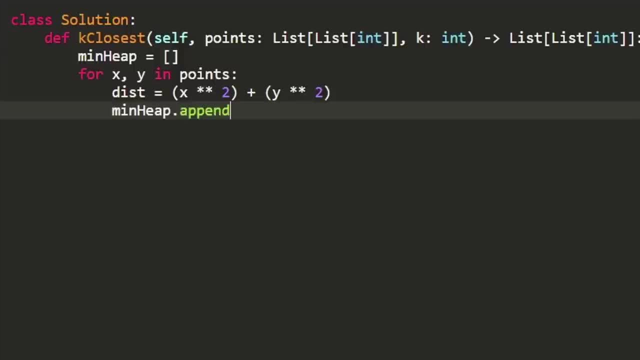 very common data structure that comes up. There's some problems where actually the entire problem itself is just using a heap, Like: okay, you know, there's some operation you're trying to do, Maybe you're trying to get the minimum value or the maximum value, Or one problem that comes up very. 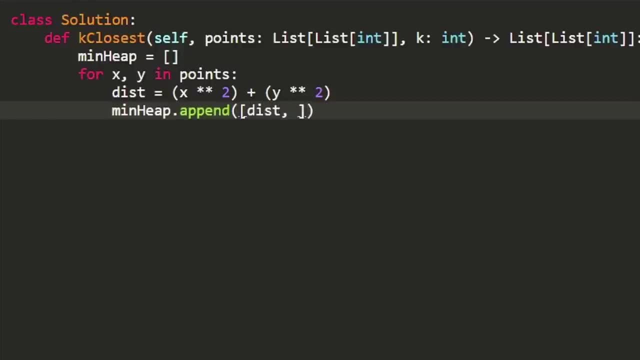 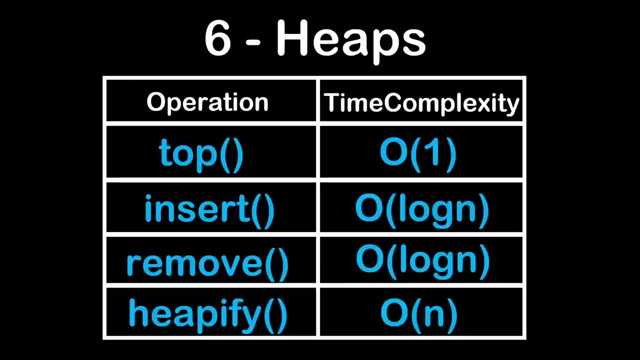 frequently is the top K values or something like that. And that's really what a heap is designed to do, Because with a heap there's two variations: a minimum heap and a maximum heap. If you were doing a minimum heap, for example, you could get the minimum value from the heap. 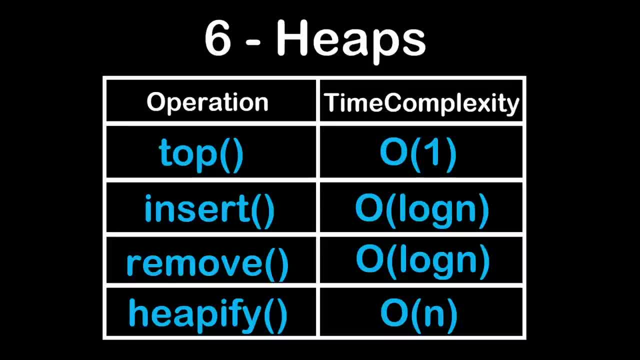 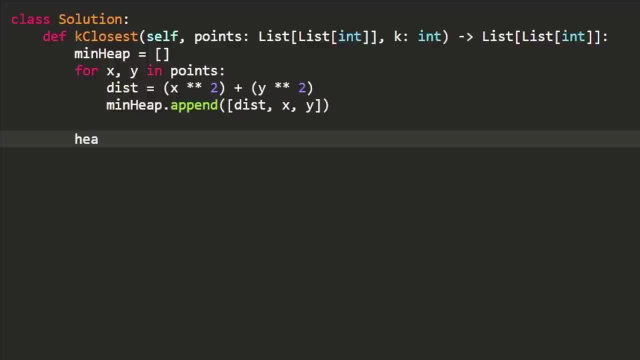 in big O of one time, which is very efficient. But when it comes to actually popping that minimum value or adding a value to a heap, that is done in log n time, which is also very efficient. One thing about a heap that I see a lot of people get wrong, and even I've had interviews where the 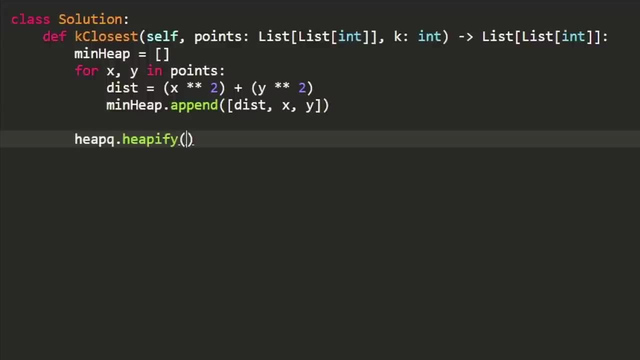 interviewer didn't know this and it was kind of an awkward situation because I was trying to explain my solution. But it's that if you're building a heap, you have 10 values or n values, let's say, and you're building a heap, you can build that heap in big O of n time As long as you have all. 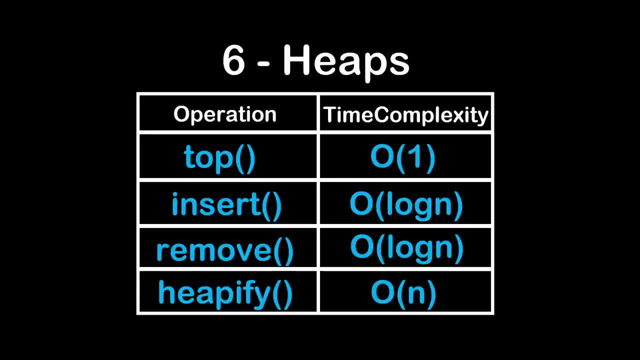 the values available from the start. you can build the heap in big O of n time. But if you're actually manually adding each value to the heap, you don't have them available all at once but you have to go through some kind of data stream to add each value to the heap. then that will take n log n. 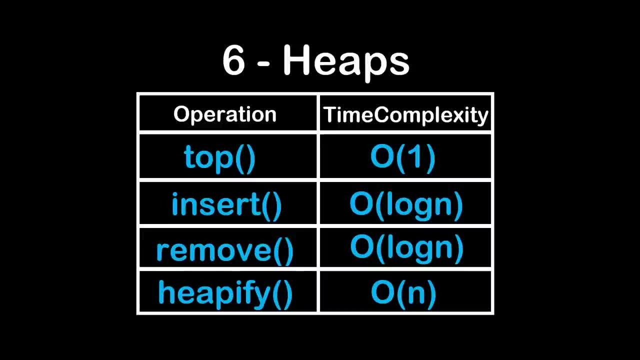 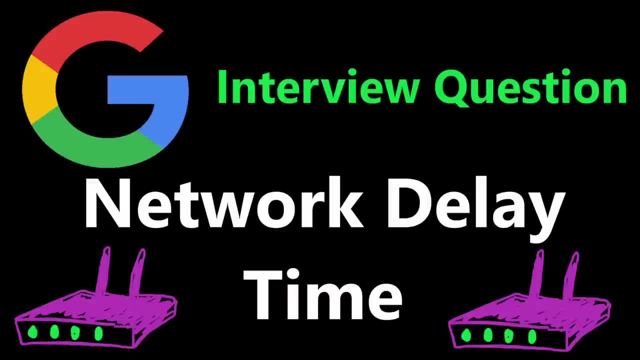 time, because adding a value to a heap is log n. If you have to do that n times, that's how you're going to get that time. complexity Heaps actually also show up in a lot of standard algorithms like graph algorithms, shortest path algorithms and things like that. So I think it's a very, very good data structure. 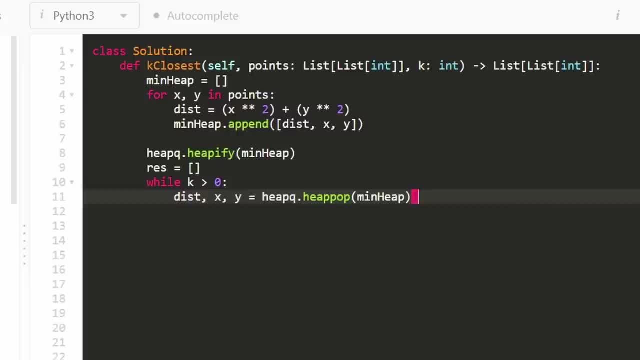 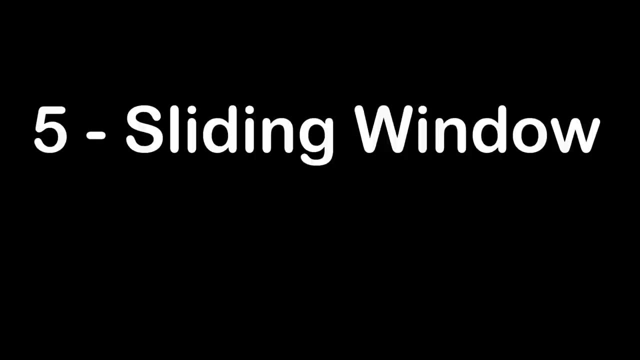 to definitely understand because the implementation is a little bit complex. but usually you don't have to implement a heap, You can just use it, and it's very easy to use this data structure. Okay, next up is sliding window. When I actually first learned this algorithm, I didn't even know. 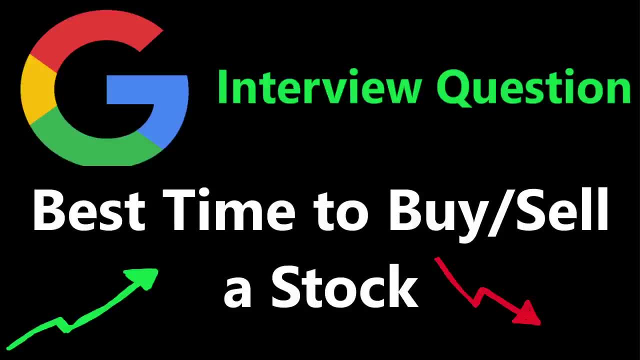 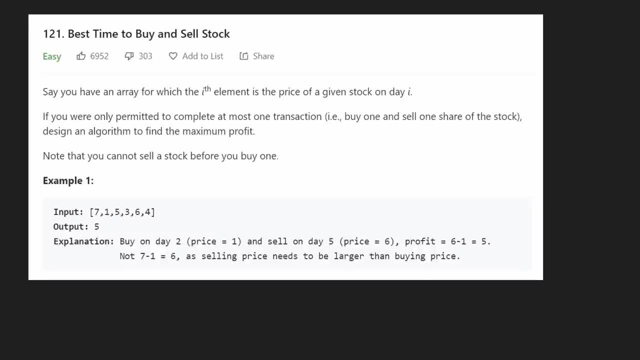 it was a standard algorithm. I was just doing some leak code problems. I couldn't figure out the problem, so I looked at the solution. Okay, there's this algorithm where you use two pointers to iterate through an array, and I remember thinking, wow, this is a really clever technique. If only I had known that it's actually. 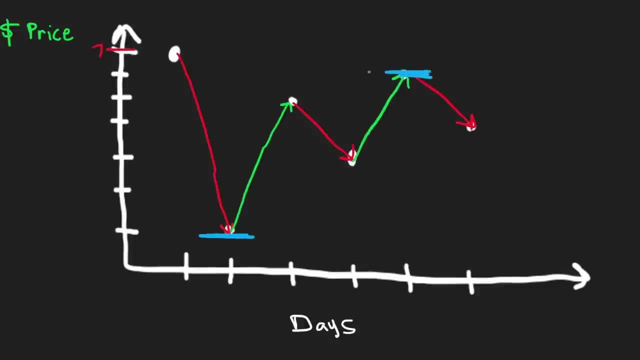 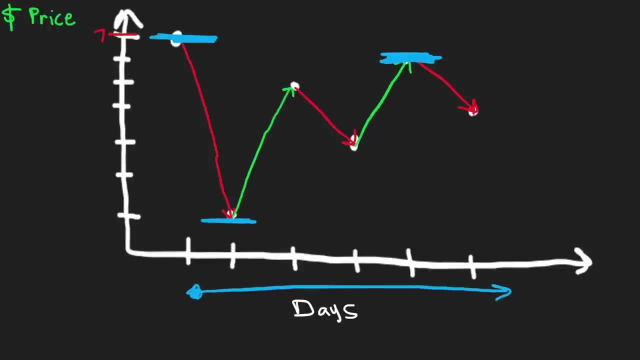 a very standard algorithm. it would actually have been easier to understand, because this is the type of algorithm you can memorize and then apply it in many, many different places. The idea is usually that to solve some problem you have to iterate through an array n times. So if you have to do 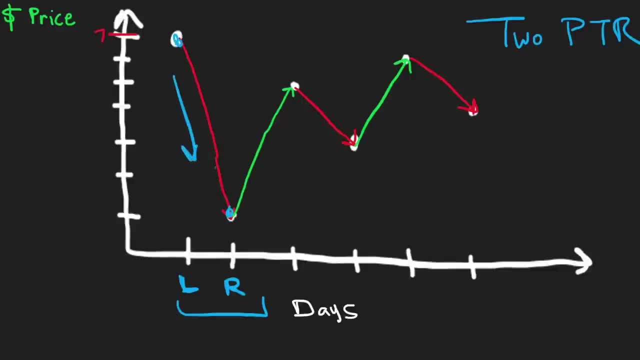 that n times the overall time, complexity becomes n. But there's a lot of problems where you can have two pointers and then use them kind of intelligently and in that way you only end up iterating through the entire array once. Well, 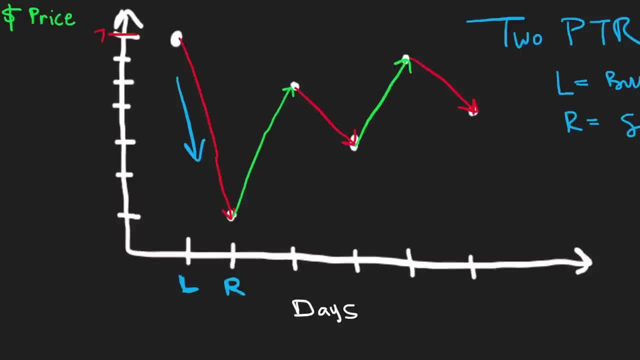 twice if you count the two pointers. but that's still big O of n time. You don't have to do nested for loops With a sliding window. you just keep track of two pointers, you increment them in an intelligent way and then you get a very efficient algorithm. We've done a ton of sliding. 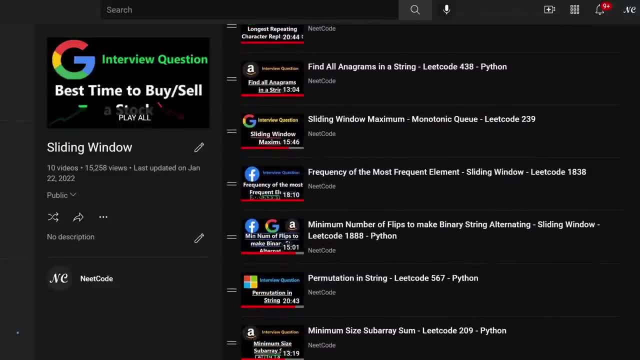 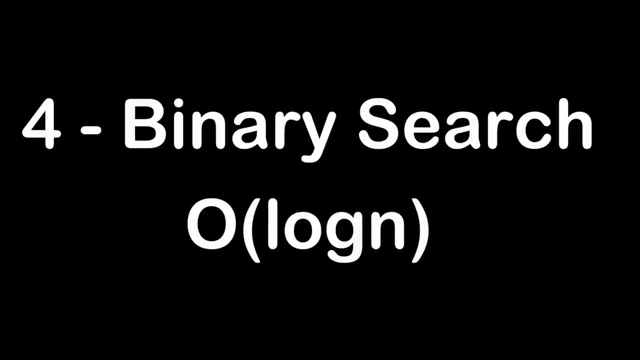 window problems on this channel, so definitely take a look at the sliding window problem If you want to see some examples. the next algorithm is going to be binary search. I think every CS major will learn this algorithm and usually think it's pretty simple, at least. 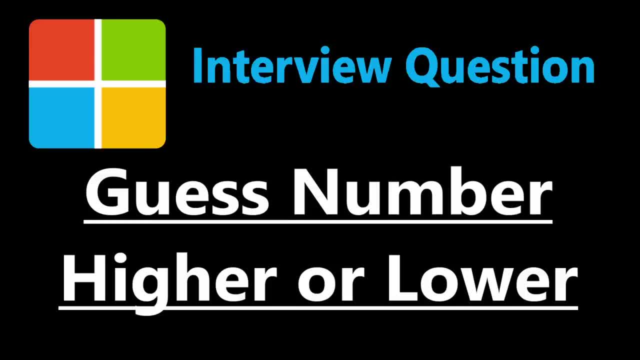 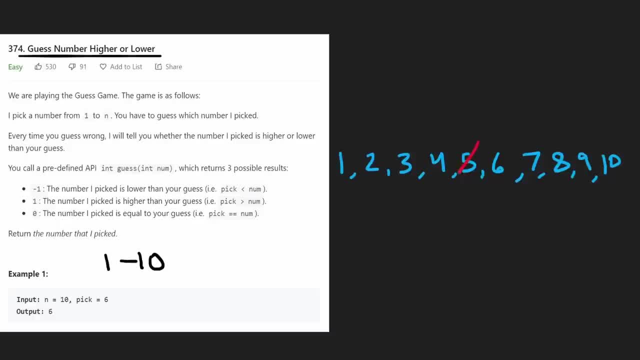 conceptually right. The whole idea comes from. you know if you were guessing a number between one and a hundred and you got some kind of feedback right, Like if you got the wrong answer, you knew if it was too high or too low, Of course, if you were guessing between one and a hundred. 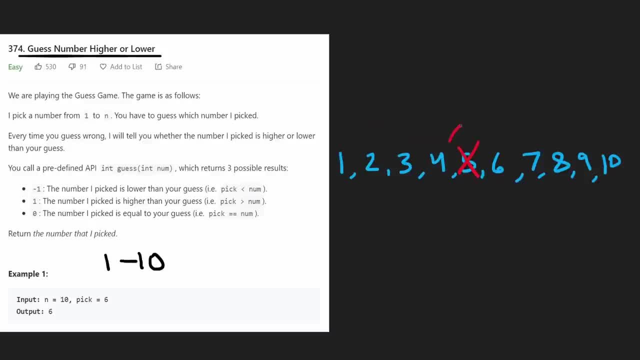 you would guess 50, because if it was too big then you would eliminate all the numbers that are smaller than 50. If it's too small, then you'd eliminate all the values larger than 50, and then just continue to do that. Just take the halfway point between whatever you're trying to. 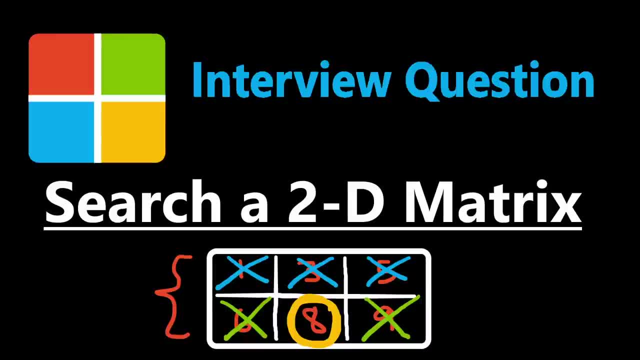 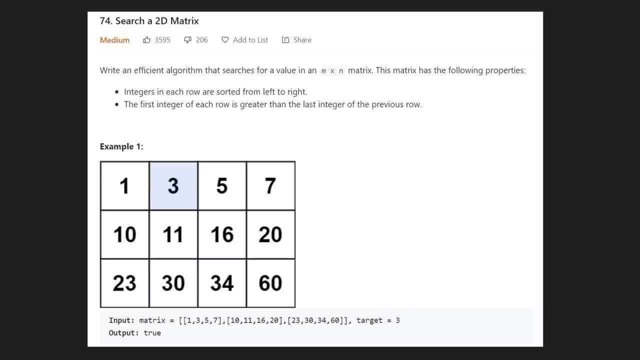 determine. So in that sense it's a very simple algorithm. Usually binary search problems are really obvious that you're supposed to use binary search. You're given some kind of array and you have to search for a value. Usually you can search for that value in big O of n time which you might. 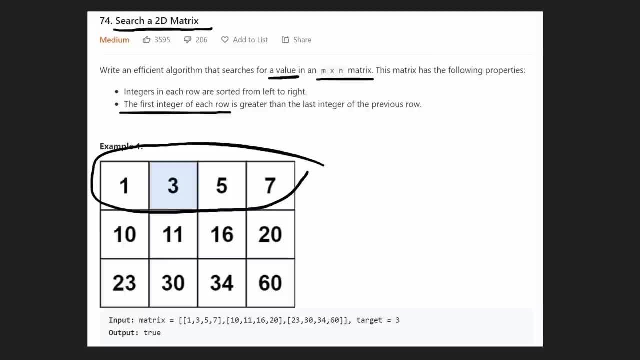 think is efficient. but if there's a more efficient algorithm using binary search, log n is actually a lot more efficient than big O of n, which is why binary search is, you know, an important algorithm. But there's also a lot of problems that are easy once you know that you're supposed. 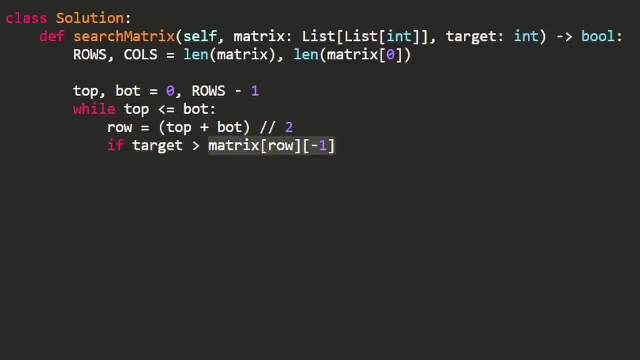 to use binary search. but it's not obvious that you are supposed to use binary search. Sometimes there's a lot of data structures involved. There's a lot of things going on. You might think it's a sliding window problem, but in actuality it's a binary search problem. So I think that's kind of. 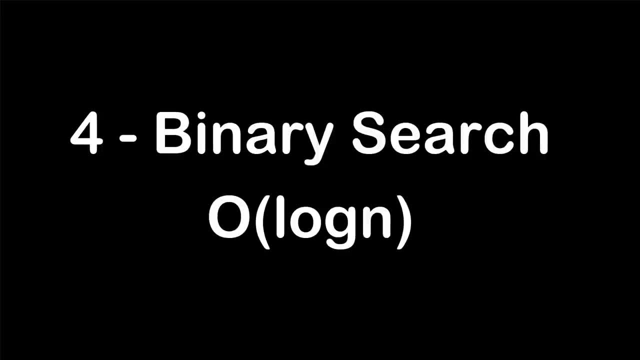 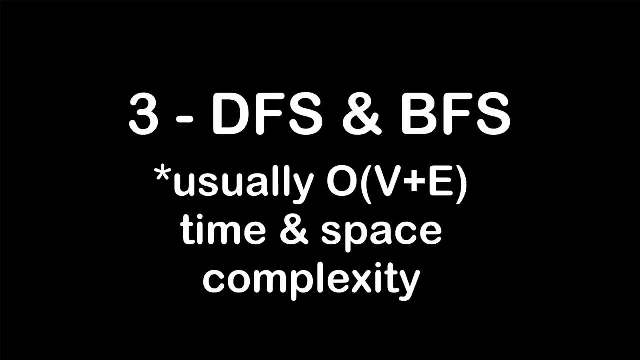 the hard part about binary search. Sometimes even identifying the problem needs binary search. We've also solved a lot of binary search problems on this channel, if you want to take a look at the playlist for that. Okay, next up is going to be actually two. 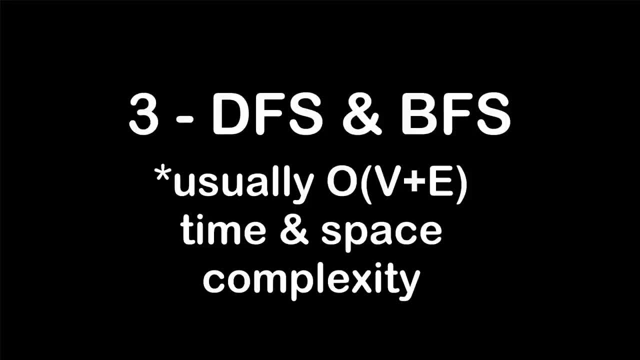 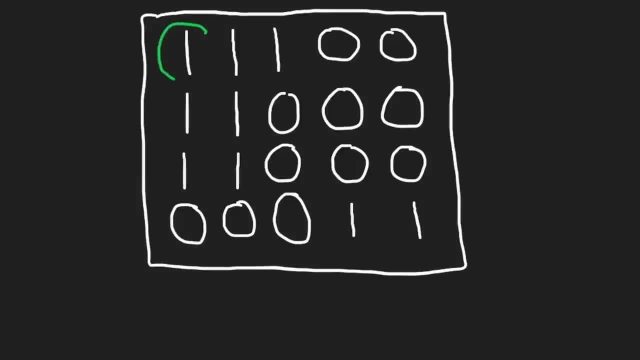 algorithms that are very similar: Depth-first search and breadth-first search. These are two incredibly common algorithms- probably the most common algorithms you'll use in coding interviews- because they can be applied in so many different places. They can be applied to trees, but they can also be applied to general graphs, whether it's a 2D matrix. 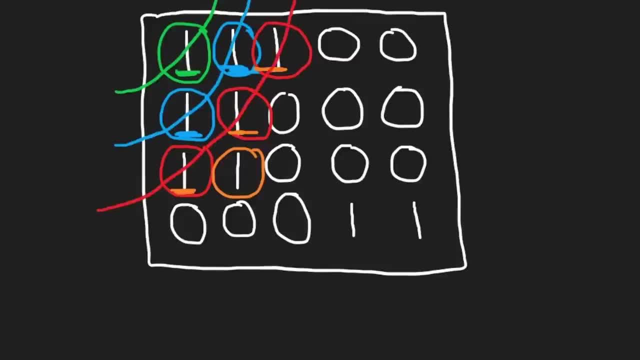 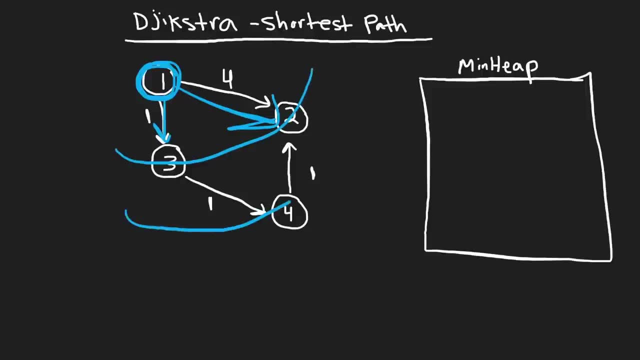 type graph or a graph of nodes and edges, And DFS and BFS are actually the building blocks for more complex algorithms, things like Jijkstra's algorithm shortest path, Kruskal's Prim's algorithm, Bellman-Ford right. Most graph algorithms build on top of DFS and BFS. So if 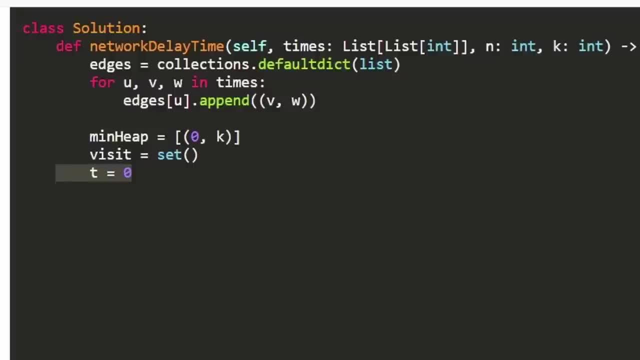 you have a very good understanding of DFS and BFS, you can actually solve a very large number of problems. And I would say, if you can get to the point where you can write a DFS algorithm or BFS, in your sleep, you're going to be in very good shape for coding interviews, because these are 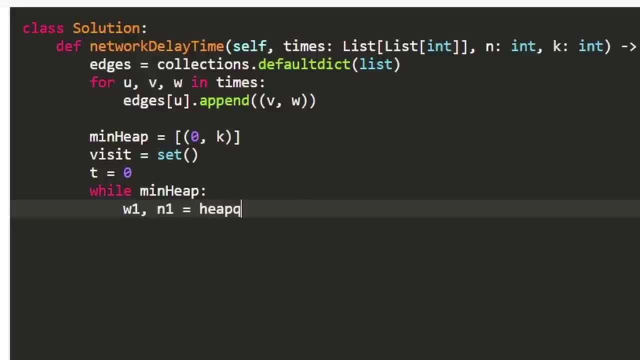 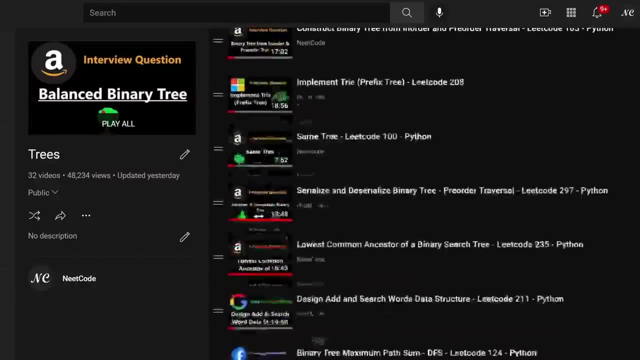 very standard algorithms. Once you've written them so many times it becomes like second nature, But when you're a beginner these algorithms can be pretty daunting to learn. We do have a trees playlist and a graph playlist on the channel if you want to practice some DFS or BFS. 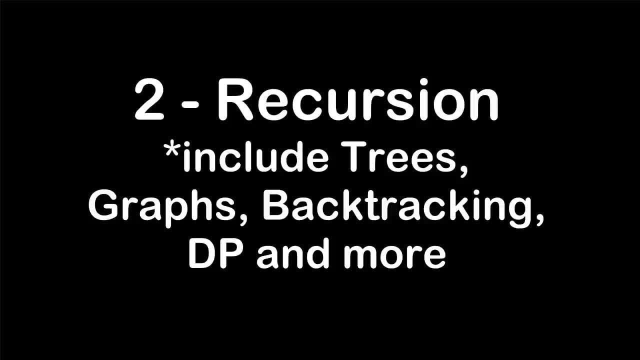 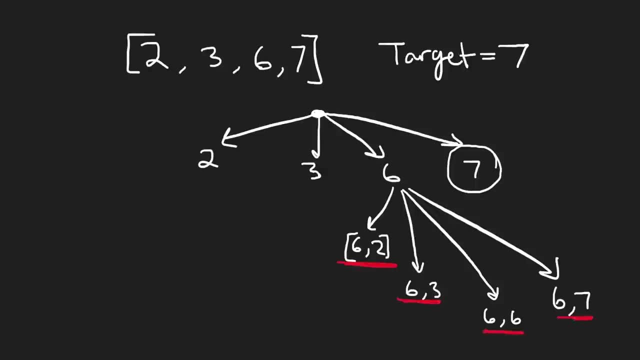 Okay, next up is recursion. Recursion was super difficult for me when I learned it back in college, but now it's actually very intuitive, Just like DFS and BFS. recursion is applied in so many places And it's also used in graphs, as well as many other categories like backtracking, sometimes with dynamic programming. 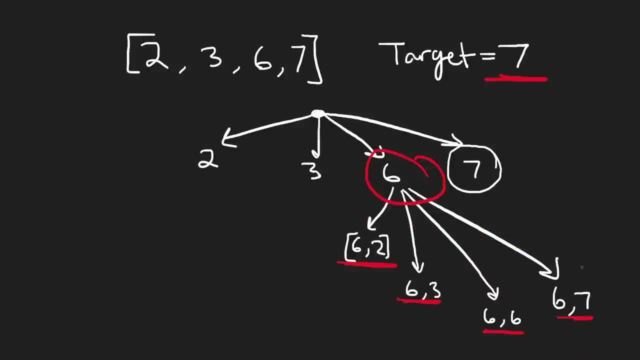 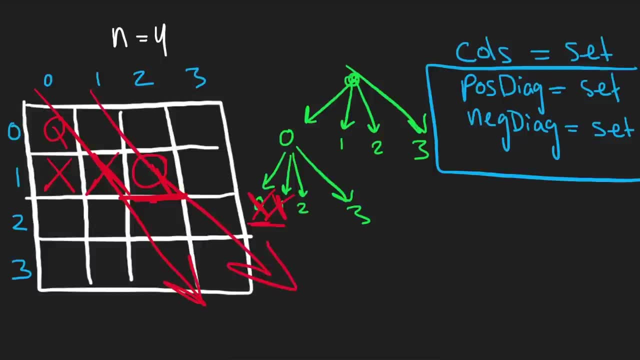 if you're talking about the memoization solution and in so many other ways, Recursion is just a huge category. I don't know how you would even prepare for coding interviews if you didn't know recursion, And I definitely recommend it. And if you're a beginner, you're going to be able to. 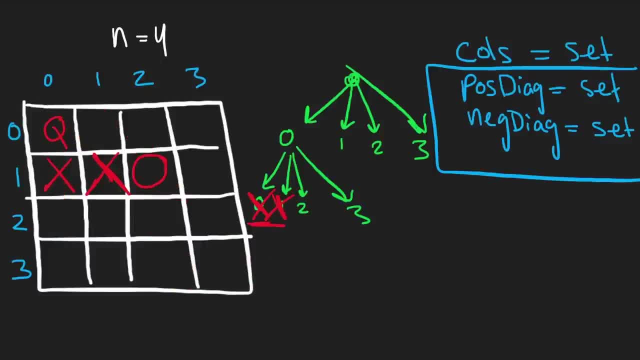 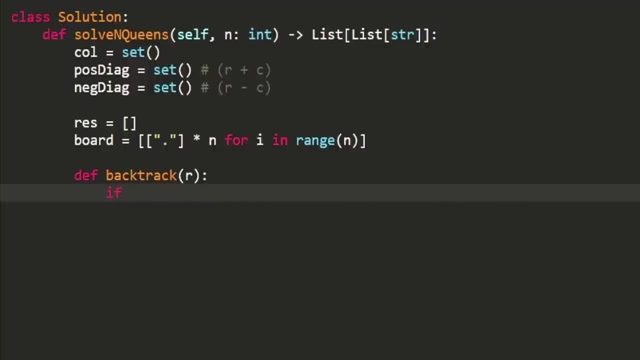 getting pretty proficient with recursion. You definitely want to have a good understanding of the base case, the recursive step and just the general idea of what's going on with recursion. You should understand that recursion does take extra memory to do. It's not free. You should. 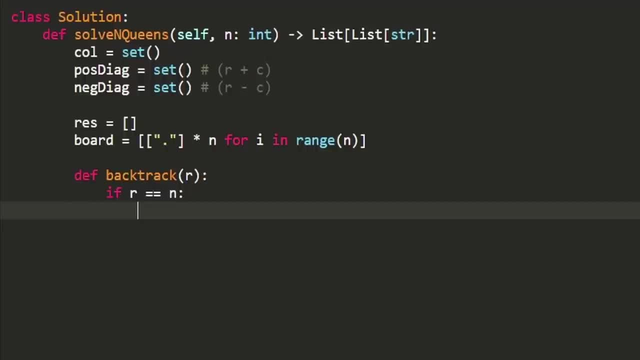 understand what's going on with the call stack as you do recursive algorithms, And I think this category is probably one of the most difficult for people to learn. I think recursion is the reason why people think graphs are hard, trees are hard and so on, And I think it's a really 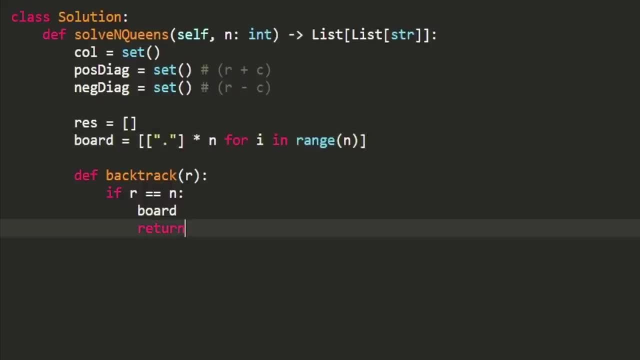 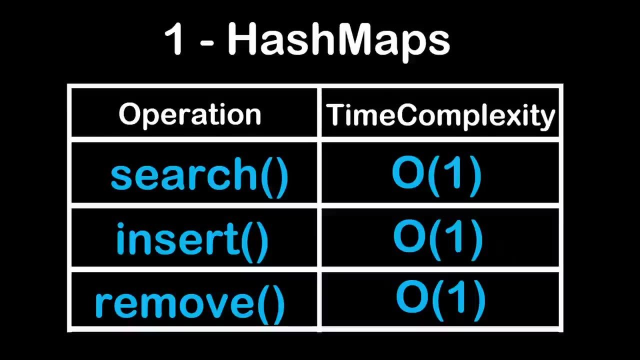 backtracking is hard, It's usually because they don't have a very good understanding of recursion. Okay, last up, the number one pattern I think you should understand for coding interviews is definitely hash maps. It's the most simple thing on this list, probably, but it's also the most. 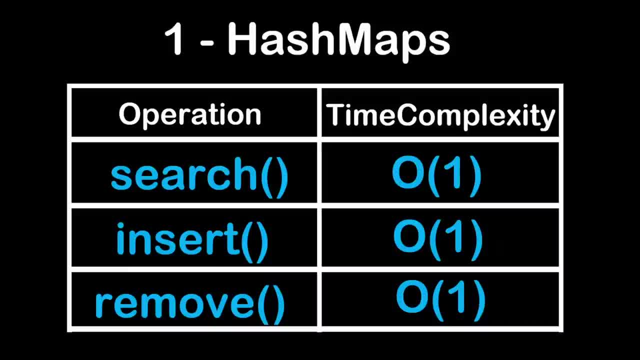 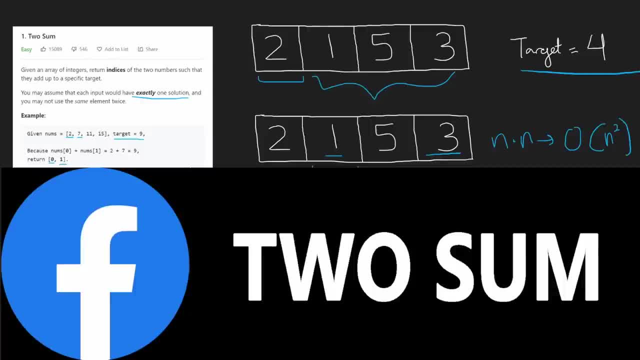 common. There are so many problems that can literally just be solved by using a hash map. The famous problem is probably twosome, because instead of iterating through the entire array to search for a matching value, we're going to have to go through the entire array to search for a. 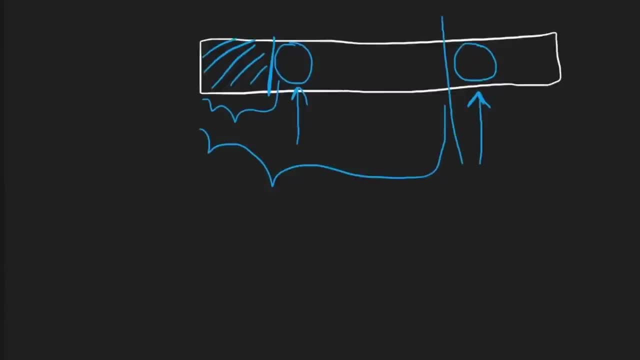 matching value. So if you use a hash map, then you solve it efficiently. And the important thing to know about a hash map is basically that every operation that you do on it, pretty much any operation at least, can be done in big O of one time in constant time. Now, technically that's. 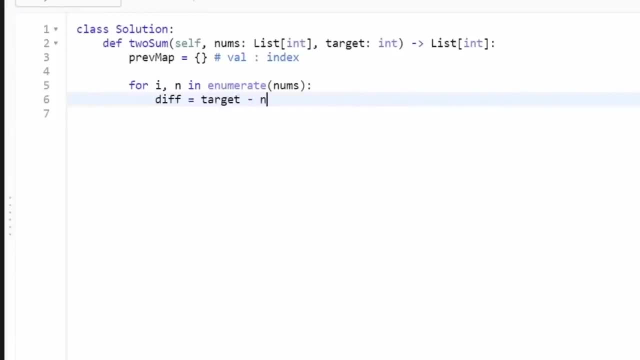 not true in that technically it's amortized because there's a lot of different ways to implement a hash map under the hood. But basically on average it'll take big O of one time and usually 99% of the time. 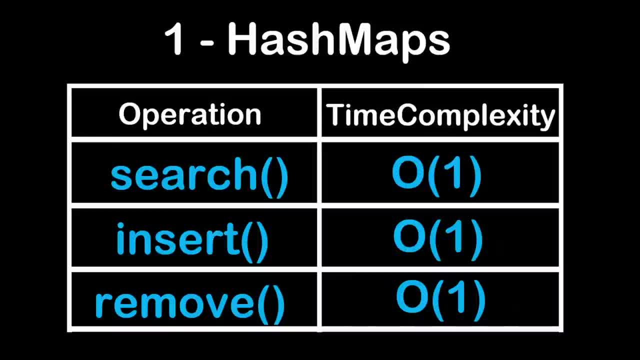 In real interviews people will just say, okay, yeah, it takes big O of one time to do that in a hash map. You don't really need to get too technical with it. Adding, removing and searching for values in a hash map is very efficient And even in a lot of the other categories I was talking.